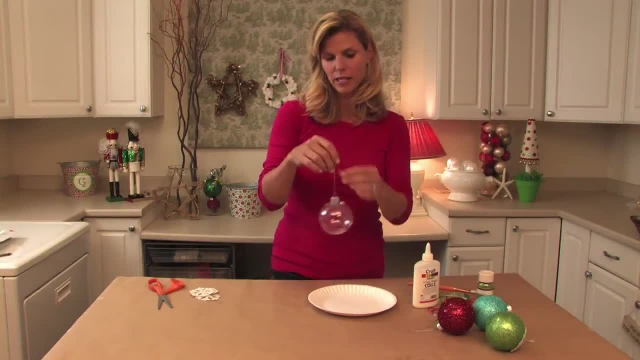 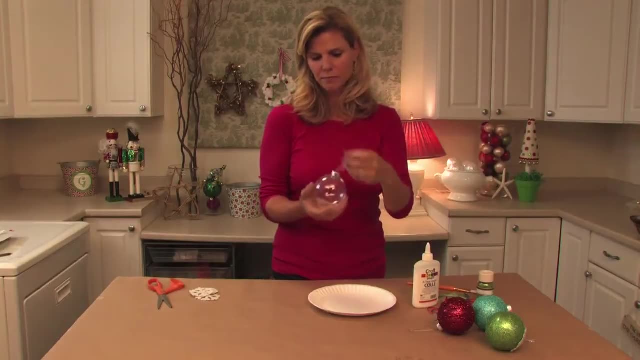 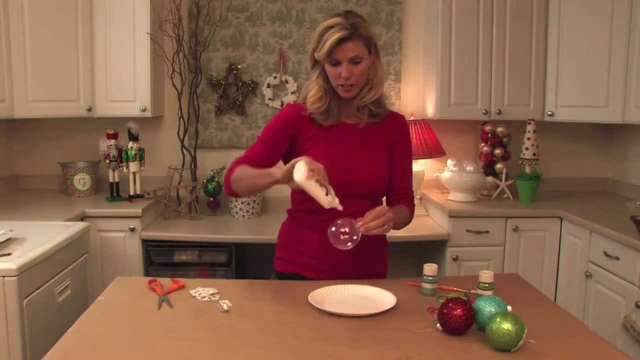 in different sizes in the craft stores and they come like this: I like the bigger size because they're just. you know, they create more of a sparkle. So what we're going to do is take the top off and set that aside. We're going to grab our craft glue and just 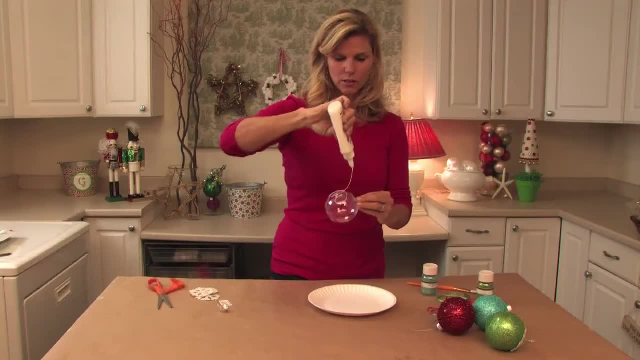 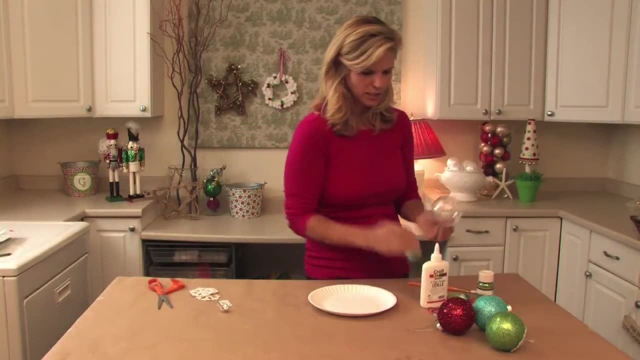 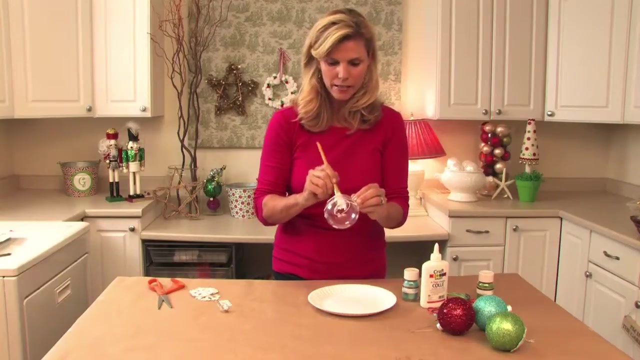 kind of put lots of glue all over the ball And the kids love this. You know they love glue, they love glitter. It's all part of the holidays- Sparkle. And then we're going to grab our paintbrush and just paint on the glue. Make sure it's. you have a liberal amount. 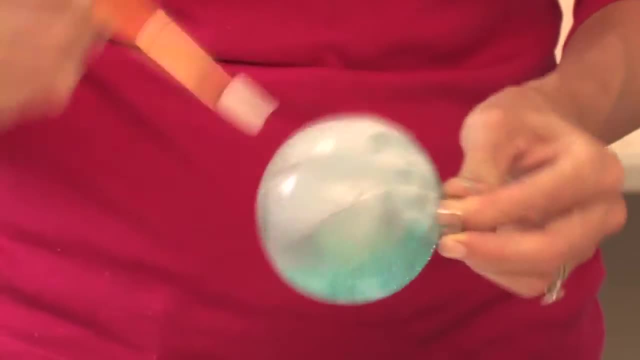 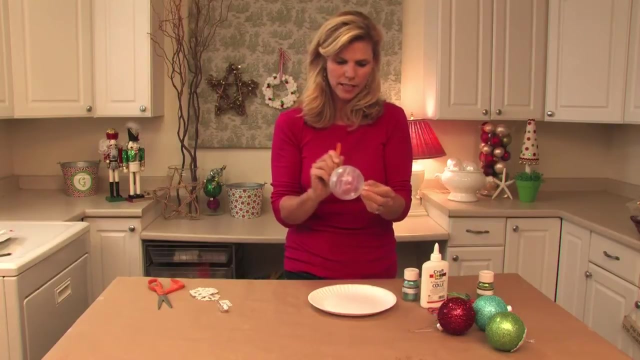 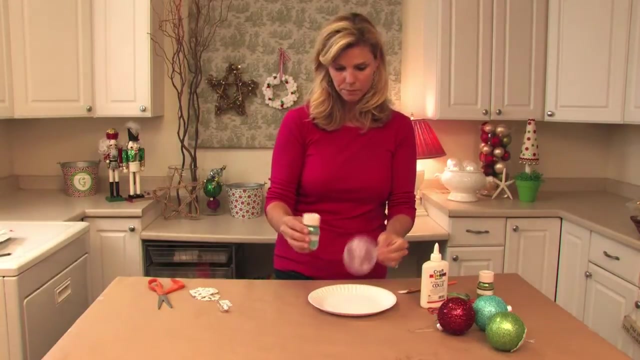 of glue And you know kids, they can never have enough glue. And remember, the perfection is in the imperfection It's. you know all about the kid's craft and how they see it and how they make it. There we go. Okay, Then we take our glitter over a paper plate and 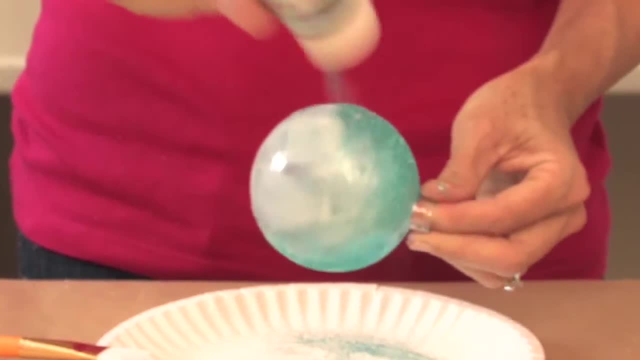 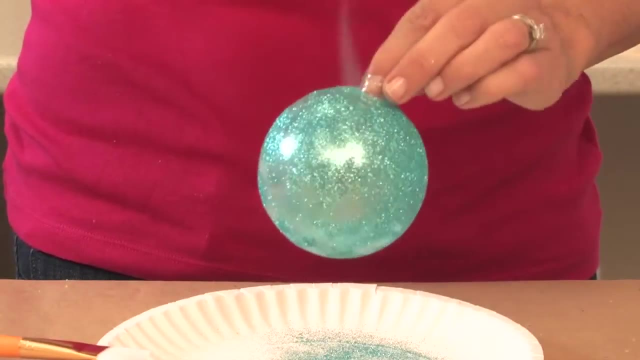 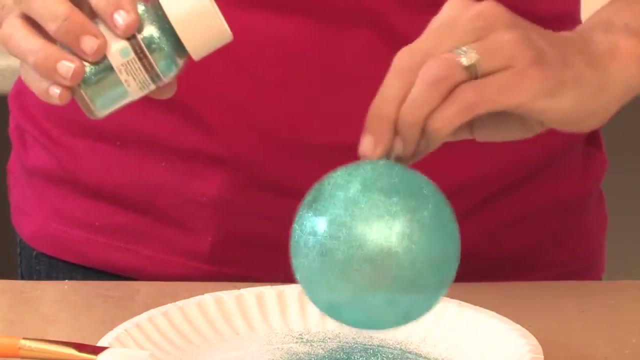 we just pour the glitter on And you just keep going and going and going until it's nice and coated. And these glitters are great. They come in so many different colors. These are a bit finer than the other glitters that you can get at the craft stores. These are really nice. 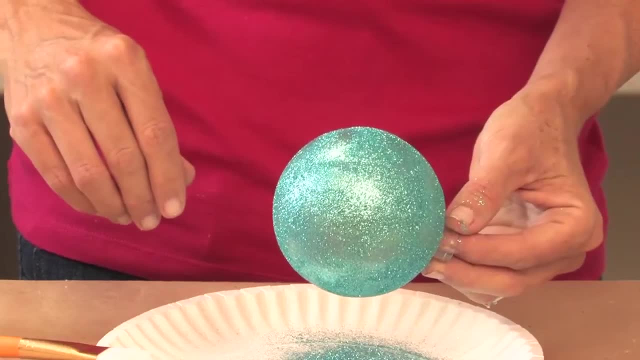 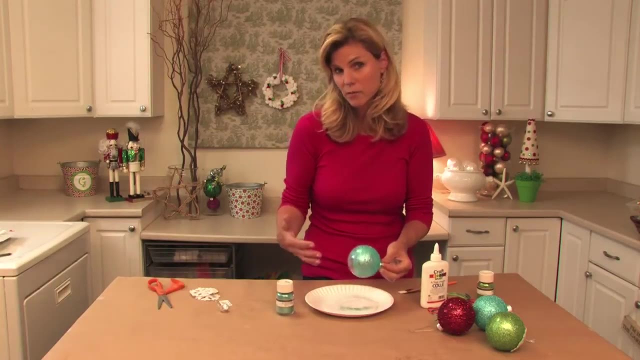 Now you just shake it off, And then what I do is, if I have a lot of glitter on the plate, I kind of take another paper plate and I put the glitter on that plate and then I reuse the glitter Because because if you have a lot of kids making these crafts, or if your kids are making them for 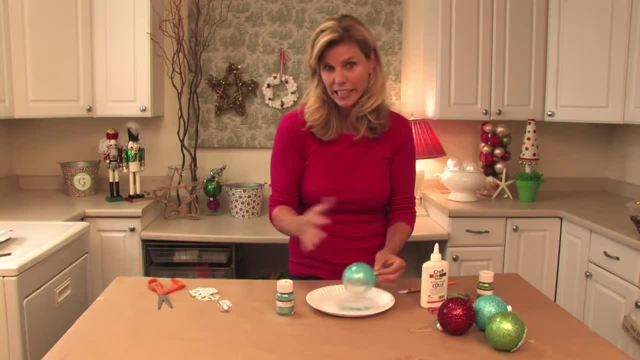 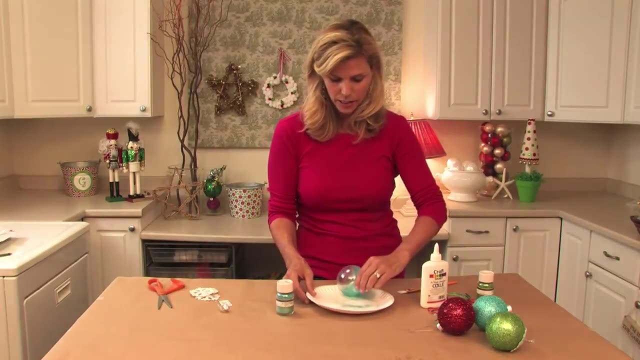 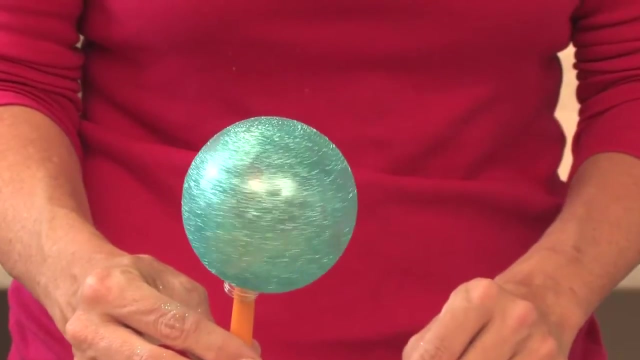 gifts, then they're going to use several. they're going to need lots of balls and lots of glitter. So once we have that covered and dried, you know what I did to dry it, I just took my paint brush and I stuck my paint brush stick in there and I stuck my paint brush, the other. 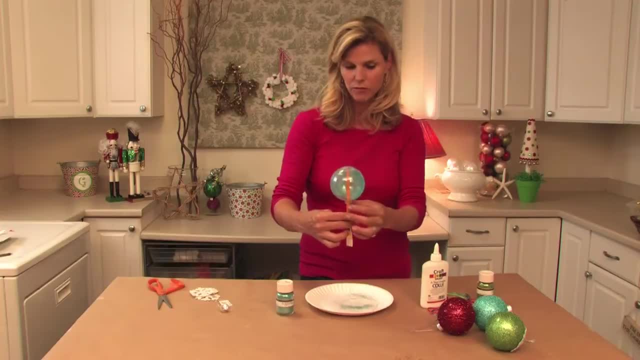 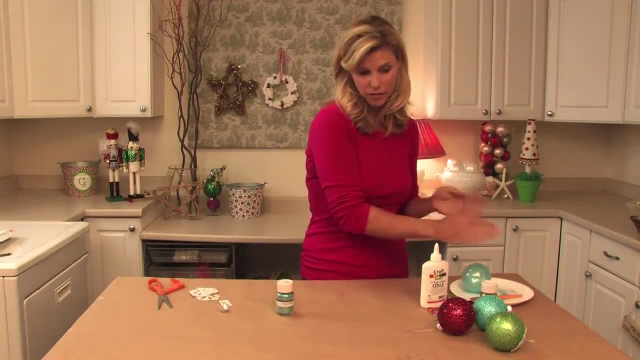 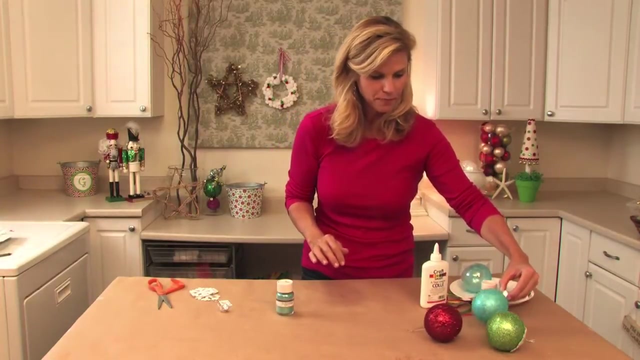 way down into a cup full of paint brushes and it kind of really dried nice and evenly that way. So once we have our ball completely covered in glitter and your kitchen is completely covered in glitter, and your kids, then we take our ball, we put our top back on and